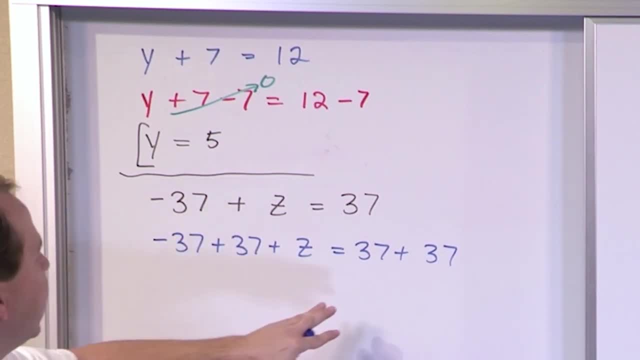 In other words, all we did was add 37 here to the left-hand side, and then, of course, we had to do the same thing to the right-hand side. The reason we're adding it is because negative 37 plus 37 is 0, and that basically eliminates everything on the left-hand side. 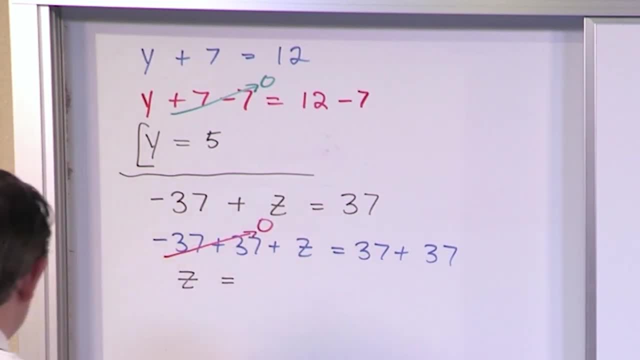 The only thing we have left is z. On the right-hand side we have 37 plus 37, which is 74.. The answer is 74.. And again, you can check it by putting 74 in for z. Negative 37 plus positive 74 is going to give you positive 37.. 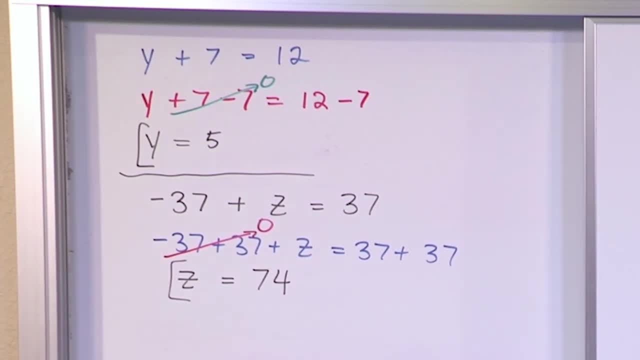 Negative, 37 for a final answer, and I encourage you to check that just to make sure. In fact, honestly, that is really one of the coolest things about algebra is that once you get an answer, you can always check it and you always know if you're right. 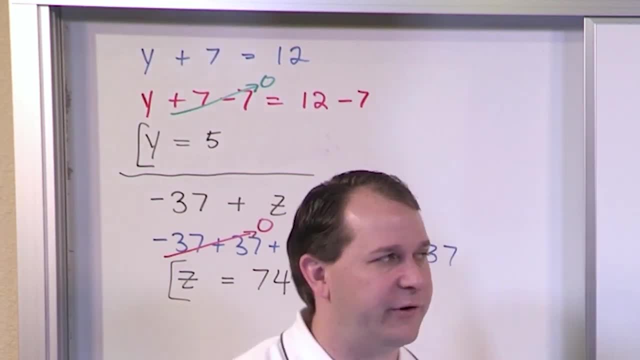 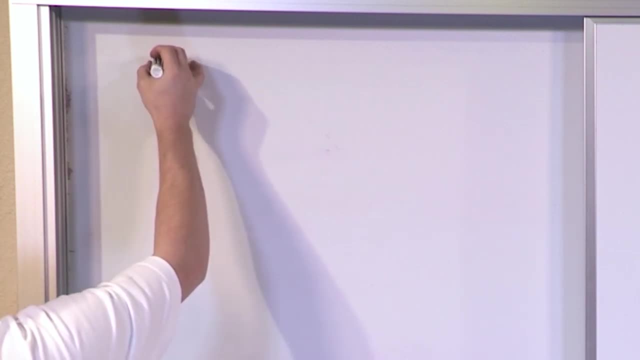 So if you get wrong answers in algebra, there's no reason, because you can always check your answers to make sure you're getting it right. All right, so let's crank up the complexity just a little bit. What if we have? 4 thirds is equal to negative 2 thirds plus x. 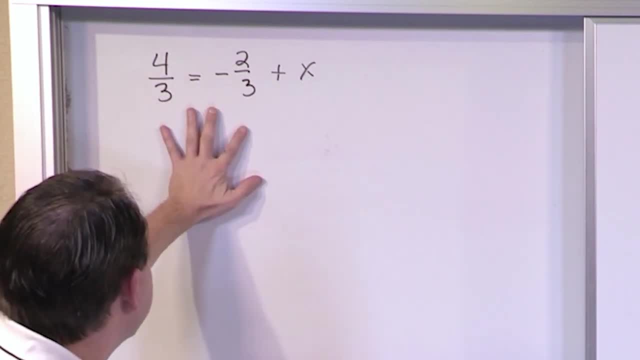 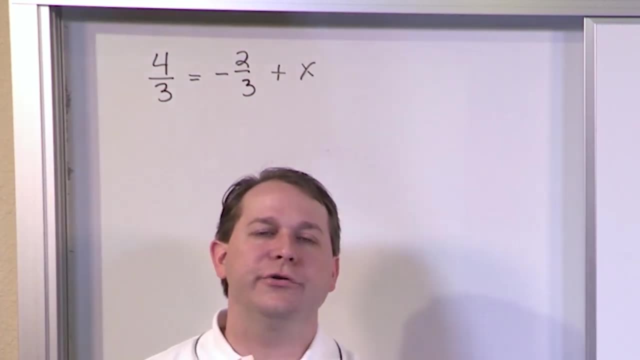 Well, there's a couple differences here. The first one is I have fractions in here, which scares off a lot of people. The second one is x is on the right-hand side. It doesn't matter where x is. All you're trying to do is get x on one side of the equal sign. It doesn't matter where it is, You just want to get it by itself. 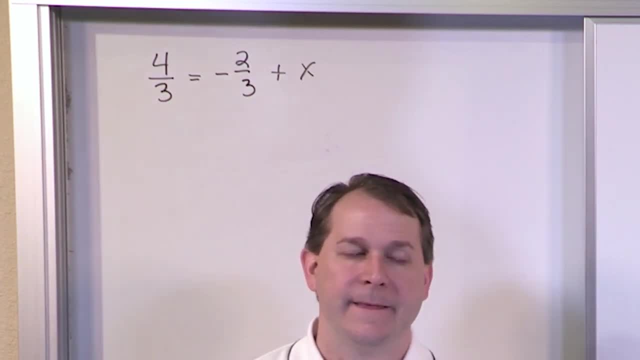 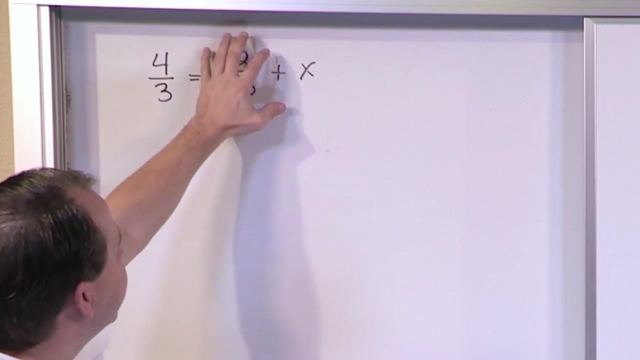 So you want to do this using the rules that we're learning here. So since this negative 2 thirds is negative, here we want to do the opposite. We want to add 2 thirds to both sides. So 2 thirds over here it's going to go away. with negative 2 thirds, It gives us 0. It's going to disappear. What we do on one side, we have to do on the other. 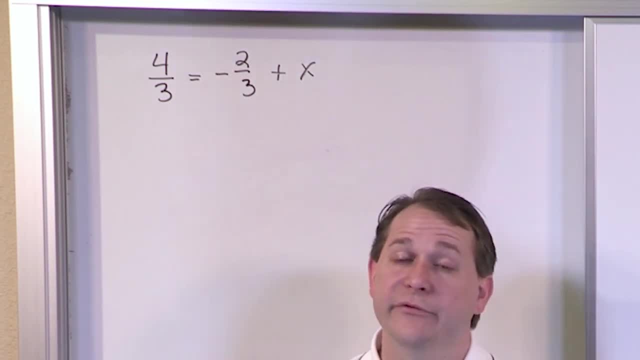 And, by the way, let me say this is a great example of why some students have problems in algebra: Because they come into algebra they kind of understand the basic idea and they get to a problem like this and they freeze up because they don't understand fractions. 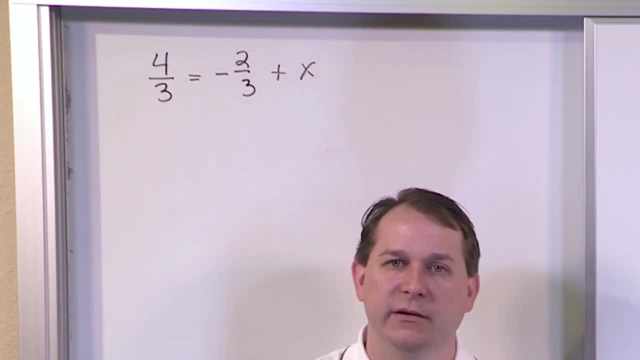 Math is so important that you build your skills one skill at a time. If you come in here and you don't understand any fractions, you don't know how to add two fractions. Math is so important that you build your skills one skill at a time. If you come in here and you don't understand any fractions, you don't know how to add two fractions. 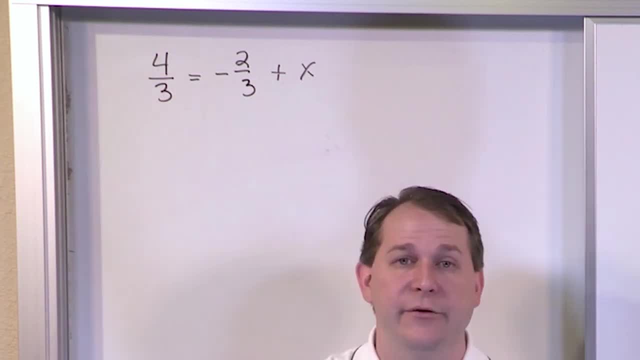 equation and then if you can't do this equation, there's going to be other things later that you won't be able to do because you can't do this, and then you kind of just it all falls apart. so it's why i take time to review fractions and i take time to review adding and subtracting negative. 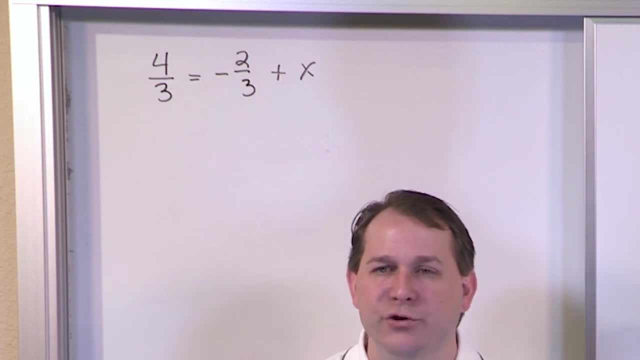 numbers and i take time to review a bunch of stuff, because if you don't get it you just cannot progress. so if this looks scary to you, if these fractions scare you a little bit, then stop, go back to the section on fractions and work those problems with fractions until you're absolutely 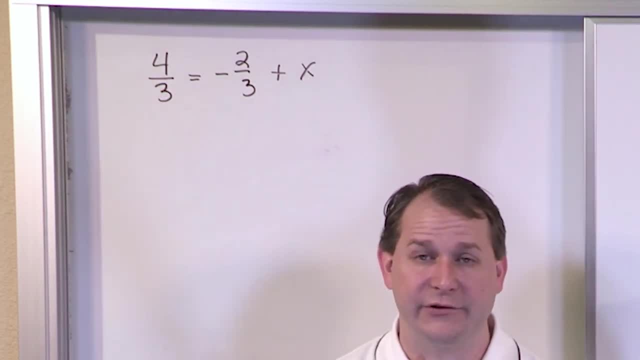 comfortable with how to add and subtract fractions and multiply and divide fractions, because it's not going to get, you're not going to, that's not going to go away in algebra, you're always going to have to deal with that. so, even though this problem looks more complicated, it's. 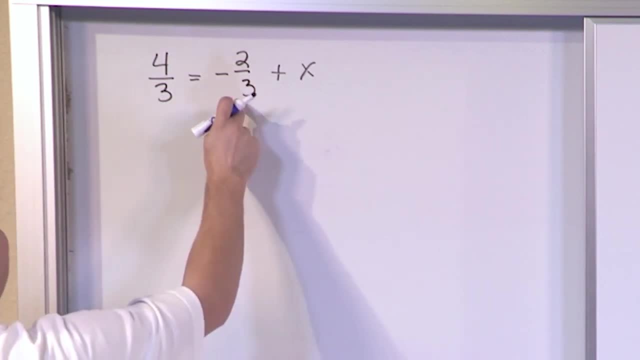 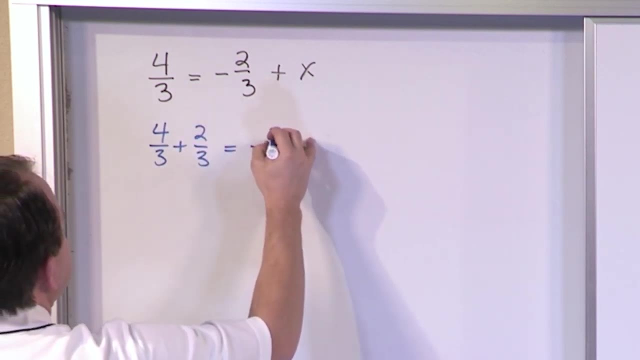 not. you're applying the same thing. what you want to do is you want to add two-thirds to both sides, so you have four-thirds on the left. you need to add two-thirds on the right. you have negative two-thirds and we're adding two-thirds to that. of course, we have our plus x. the only difference. 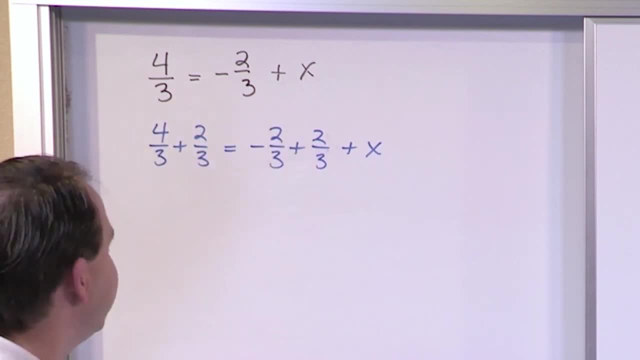 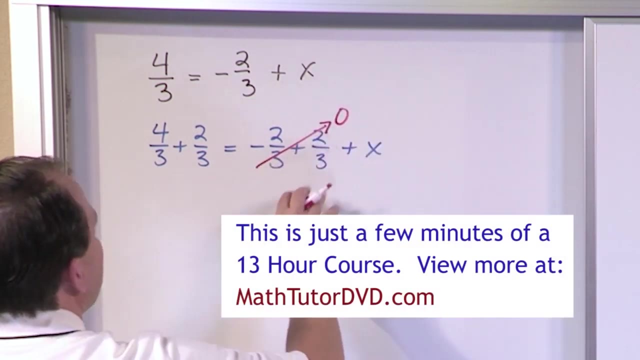 between this and this is: i've added two-thirds to both sides. and the reason i've added two-thirds to both sides is because negative two-thirds plus positive two-thirds is zero. i'm trying to get x by itself. okay, i'm trying to get x by itself. so what i have here on the left hand side, i've got. 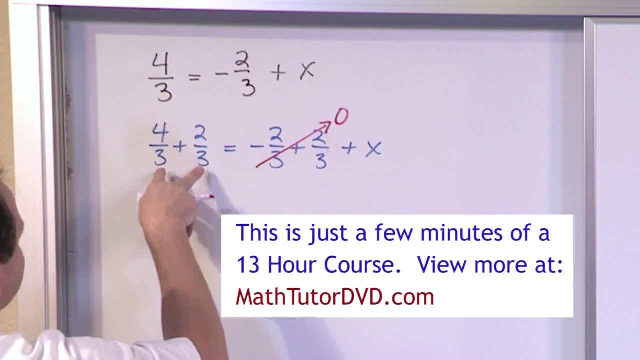 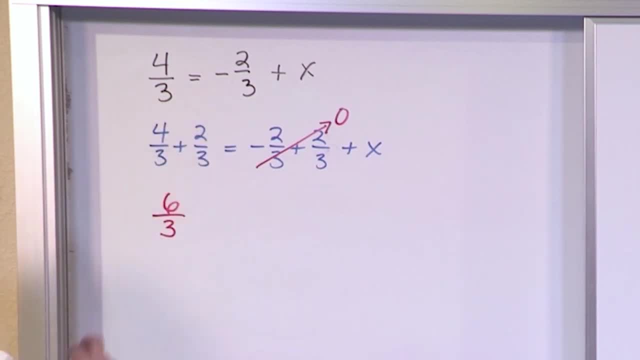 two fractions that i need to add together. fortunately, the common denominator is already here. i've already got a three, so i keep the common denominator, i add the numerators, i get six-thirds on the left, and that's all from fraction arithmetic on the right hand side. 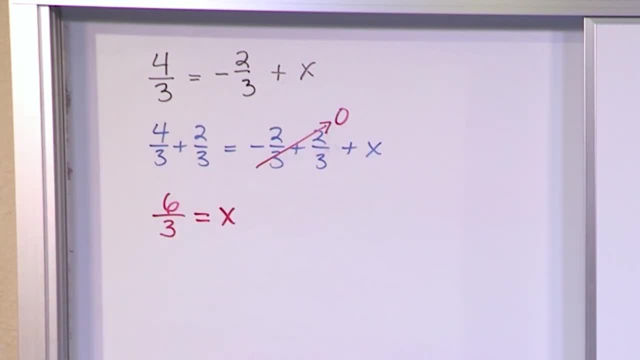 this goes away and i have x. now let me ask you this: six-thirds is really six divided by three. so what is that? so that's two. so two is equal to x. so it doesn't matter that it's two is equal to x, it's exactly the same thing as x is equal to two. you've learned that it doesn't matter if x is on. 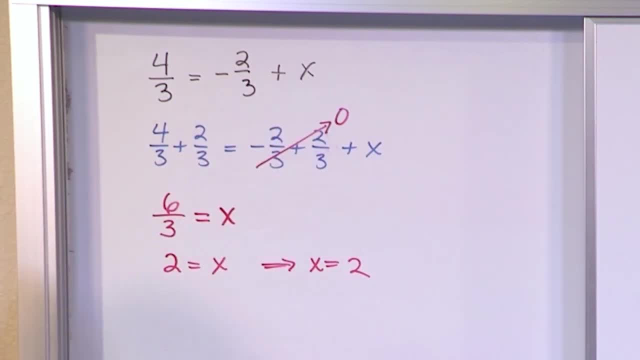 the left or the right hand side. you still just try to get it by itself, and then you have the answer. so x is equal to two. that is the answer to this problem.